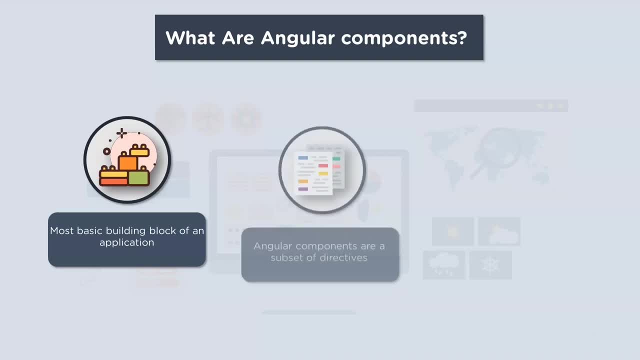 branches out into other components, creating a hierarchy, And these components are a subset of directives. Now, don't worry about what directives are, because we'll cover them later on in the series, But to give you an idea, there are three types of directives. You have the 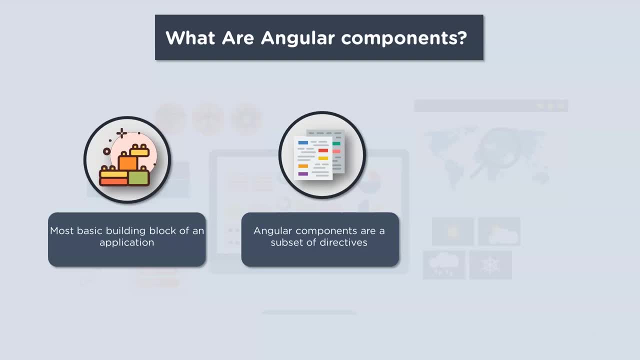 structural directives, the attribute directives and the component directives, Only one component can be instantiated per element in a template. Now, components are typically custom HTML elements and each of these elements can instantiate only one component. Now, don't worry, you'll understand. 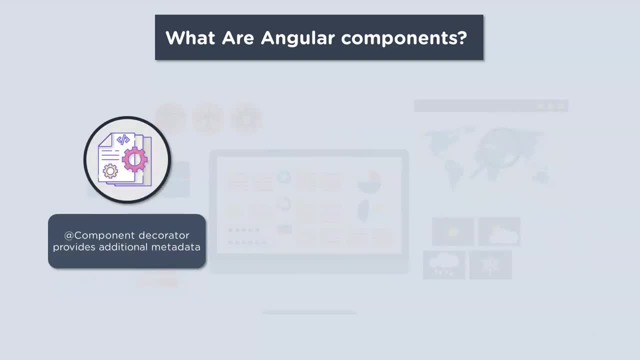 this better when I show you the demo. Nextly, a TypeScript class is used to create a component. Now. this class is then decorated with the at component decorator. Now the decorator accepts a metadata object that gives information about the component. Now. 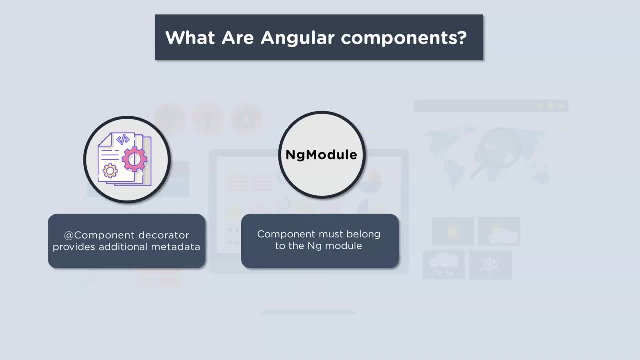 a component must belong to the ng module in order for it to be usable by another component or application. And finally, components control their runtime behavior by implementing lifecycle hooks. So this was just a brief introduction to what Angular components are. Now you will only be. 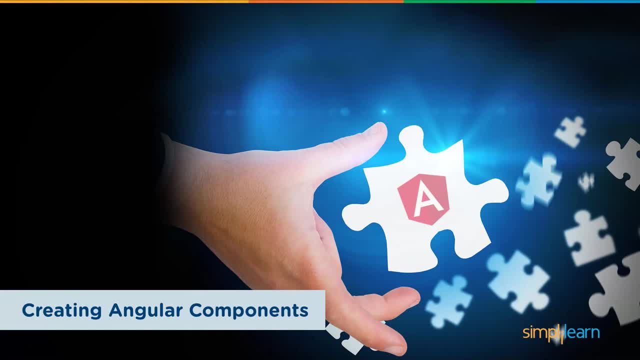 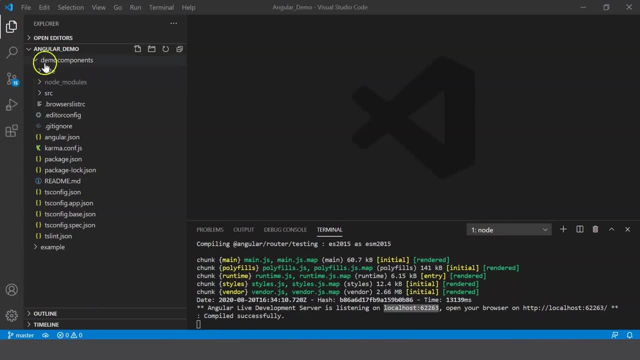 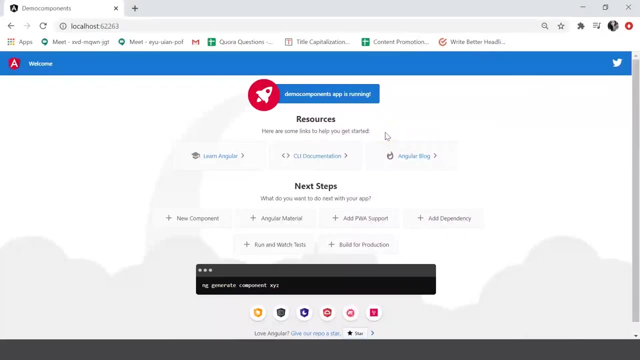 able to understand the working of components when I show it to you practically. So let's head over to a Visual Studio Code Now, here back in my VS code, I've created a folder called Angular Demo, within which I've created an Angular application called Demo Components Once executed. 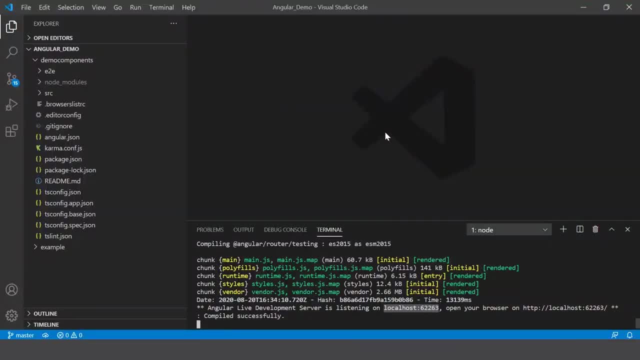 the browser looks something like this. So if you haven't watched our previous video on getting started with Angular- that is, Angular Hello World- I highly suggest you go through that video first. It helps you create your first Angular application. So now let's go ahead and create. 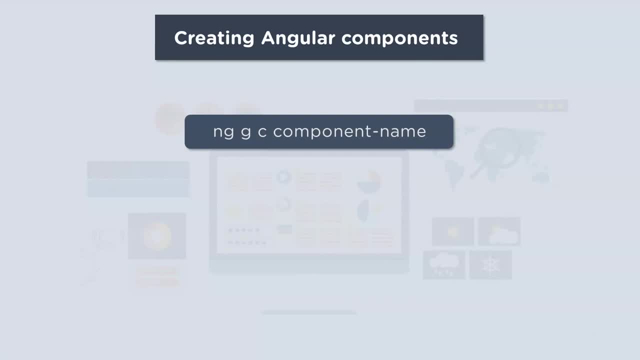 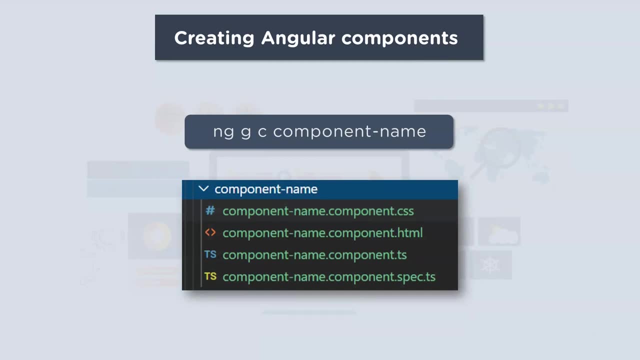 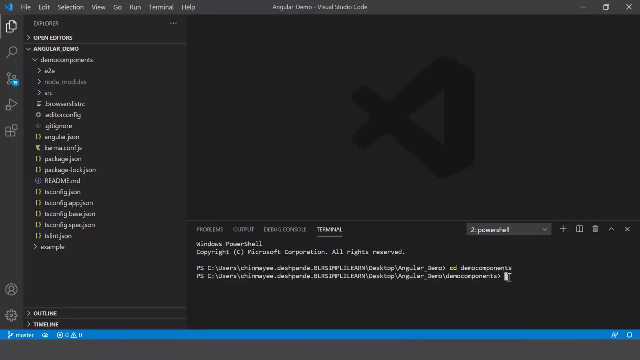 our first component. Now, the command used to create our component is ng gc and your component name. Once executed, it creates four different files. Now let's just see how this works on our VS code. Now what you can do is head to your terminal and type in the command ng gc and provide. 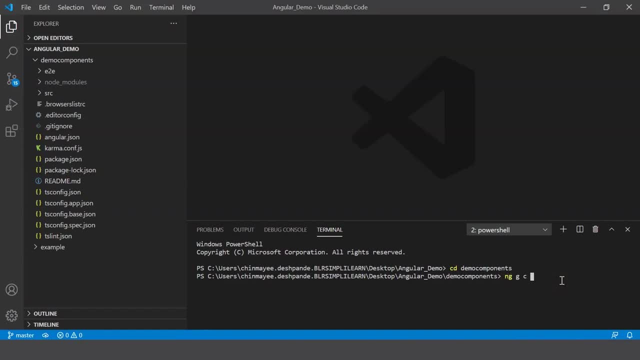 a name for your component, For example, I'm going to just call my component text component. All right, So what it does is that it creates four different files. You can see you have four different files that have been created and finally, it updates the file that is appmodulets, indicating that. 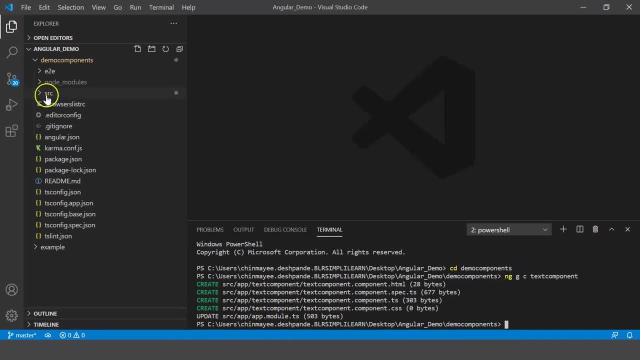 this new component has been created. So here in your source folder, within which there's an app folder, and again here you can see that your four different files have been created. First is the HTML file, wherein you can define all the code that you want for your component. 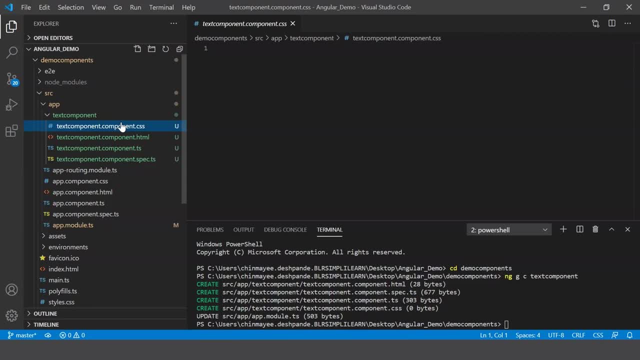 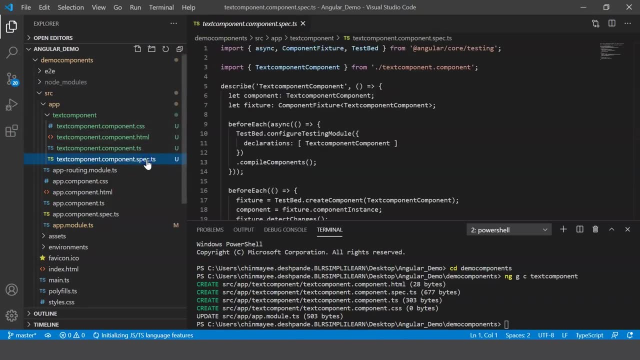 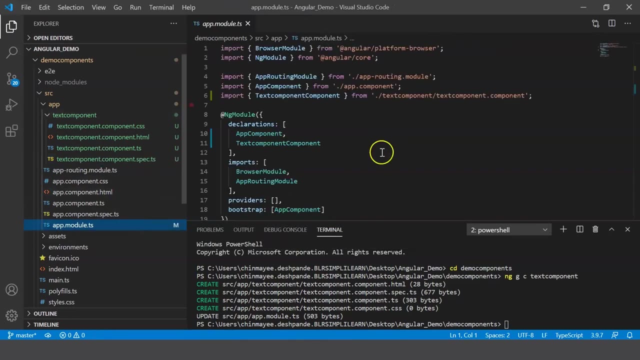 Next, you have the CSS file for your styling, Then you have the ts file, which includes the component decorator, And finally you have spects, which is basically a unit test file. All right, And then in your appmodulets you can observe that the component that you've created, 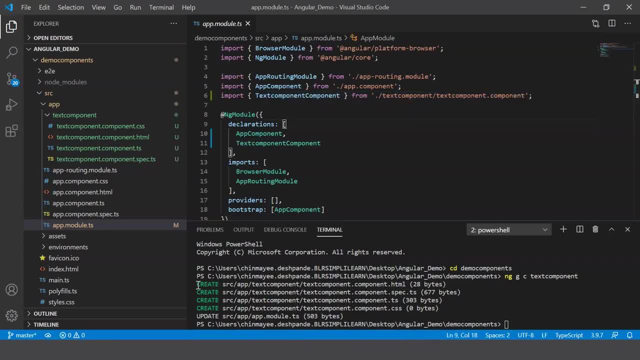 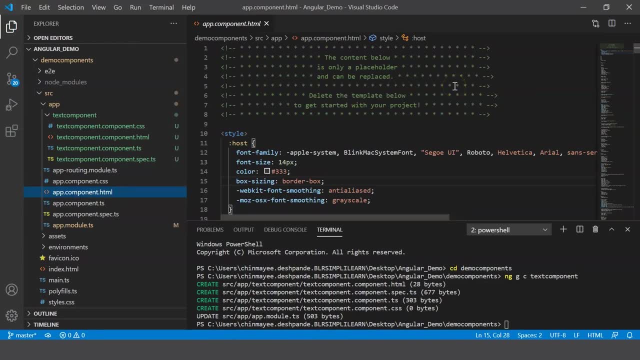 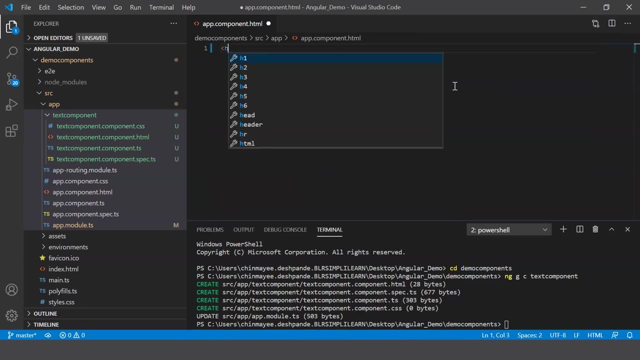 that is, text component has been imported. That is what the message conveys here. All right, Now let's go back to our appcomponenthtml. Now this basically has all the the code for your application, so let me just get rid of it and I'm just gonna display a basic. 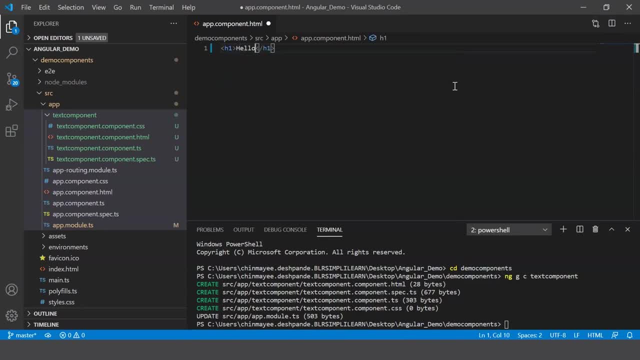 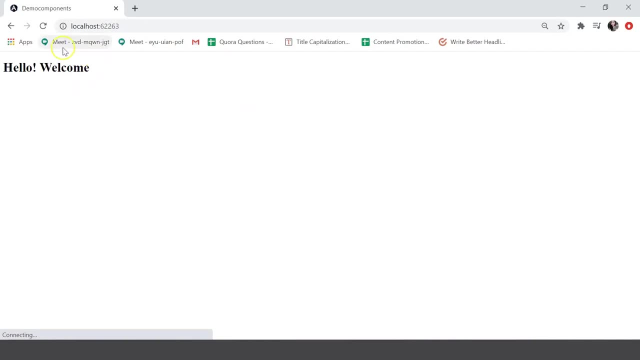 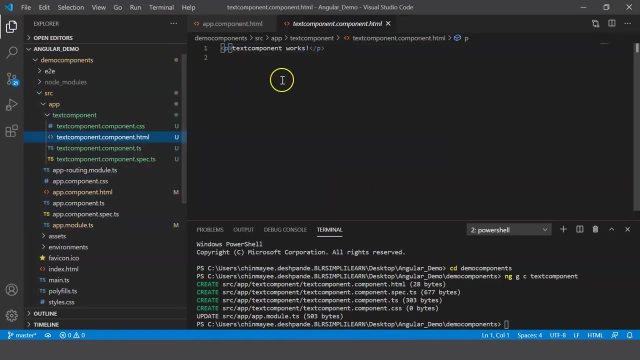 heading saying hello, welcome, all right, so let me save it and if you go ahead and look at your browser, hello welcome message is displayed. now let's go back to our component dot html file and here let me provide a message. let me say h3 and let me display a message saying: 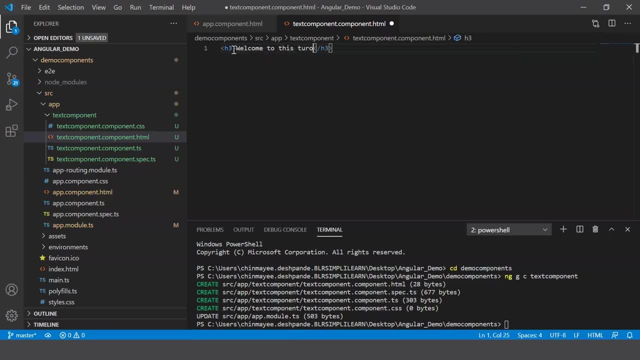 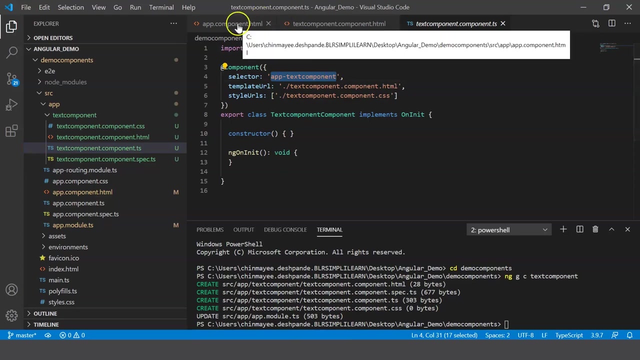 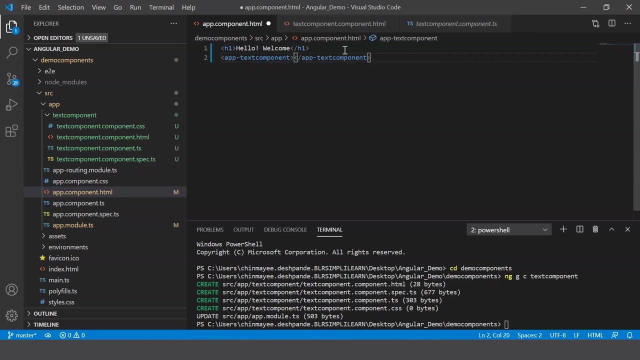 welcome to this tutorial on angular components. all right now, in your text component, dot ts file, which is your typescript file, the selector mentioned here is app hyphen text component. now go ahead and copy this and in your final component, dot html, go ahead and create your custom html tag with the selector that you just copied. now this indicates: 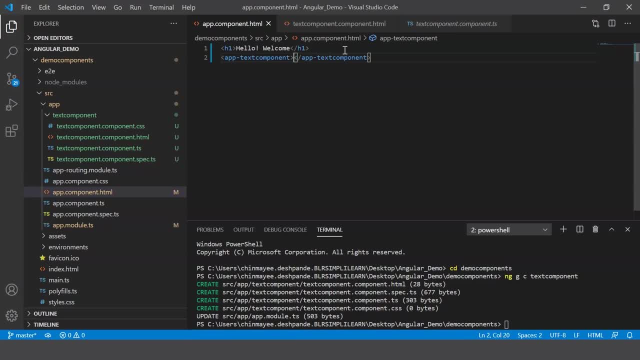 that the component that you just created, that is, the text component, is being incorporated in the final render. so what happens is that whatever is defined in the component dot html file is also being rendered in your final out output. so when I save this, let's go ahead and check our browser. you can see that the message 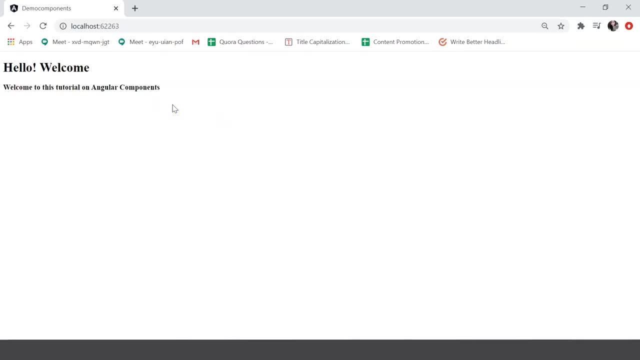 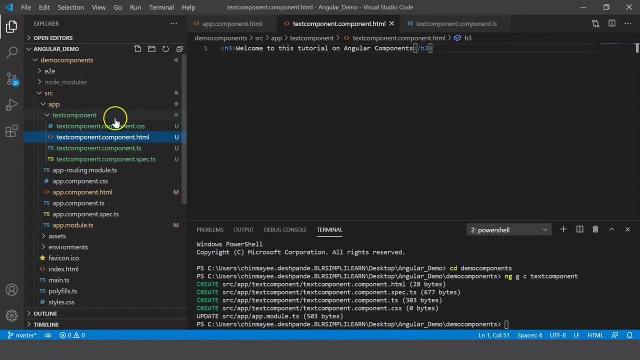 welcome to this tutorial on angular components is displayed. so this was a simple creation of a component. now for this, let's give it some styling. so here, go to your dot css file and provide some styling. say for example: here I just say text align, and then I'm going to go ahead and create a new component, and I'm going to go ahead and create a. 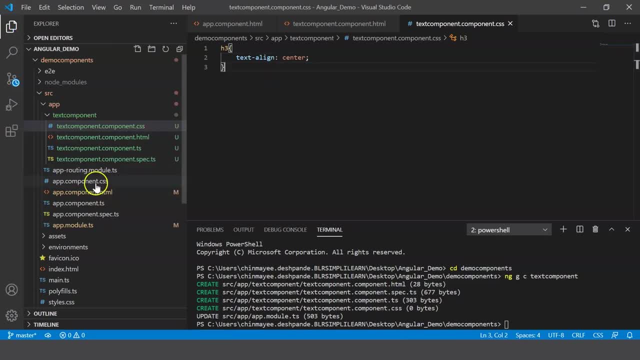 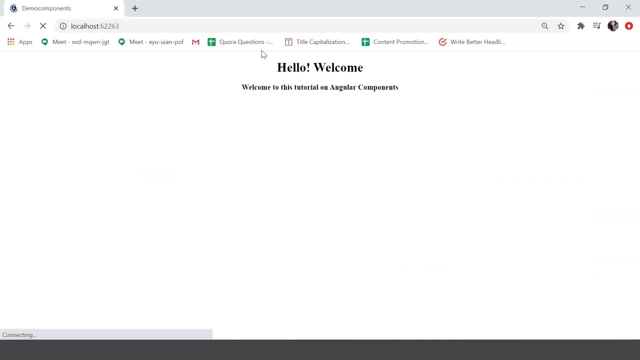 component and let me say center. and also in my appcomponentcs i'm going to give the same thing and say each one text align is center, all right, so let me save this. and there we go. now. you can also create multiple components and define the tags in the app component. now the components. 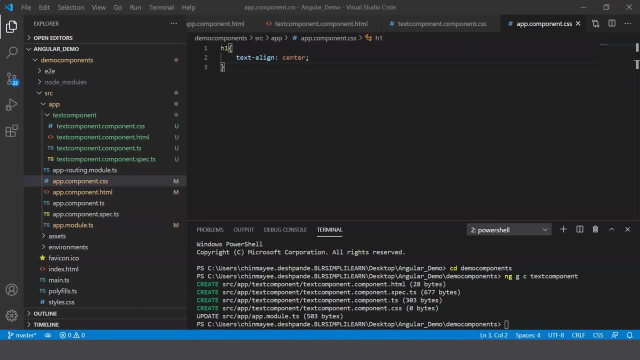 are executed sequentially. so now let's create another component, just to give you a brief insight into it. so let's start out with this. we'll begin our onlination and after that we'll go back to amazon. phaFlix- hedalic tests- någonting. 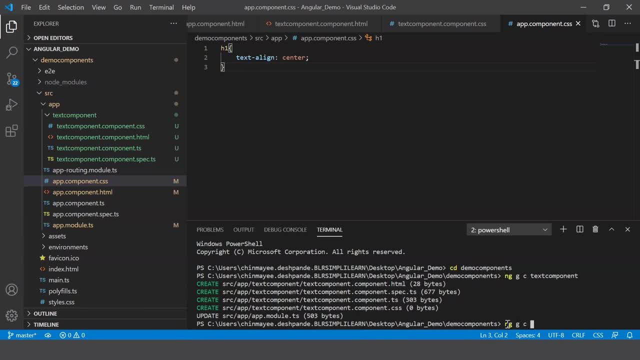 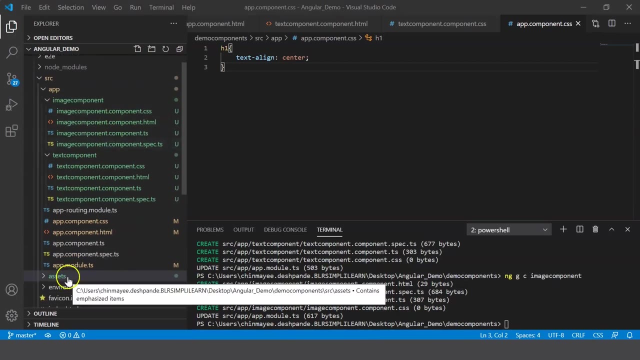 into it, Let's say ng-gc image component. Now here I'm going to be adding the Simply Learn logo, So I'll show you how that works. Now you can see that a new component has been created with four files again. So in my assets folder here I've added the logo. So what I can do is back in my 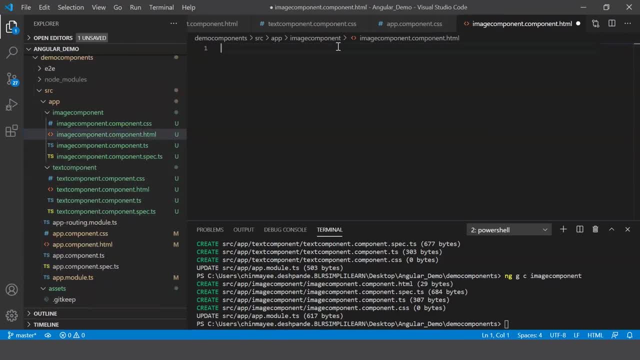 HTML file, I can go ahead and create an image tag. So first let me just display another message here, Just to avoid any confusion, And let me say: this is the image component. And then let me say: image source equals, So the source is basically assets. 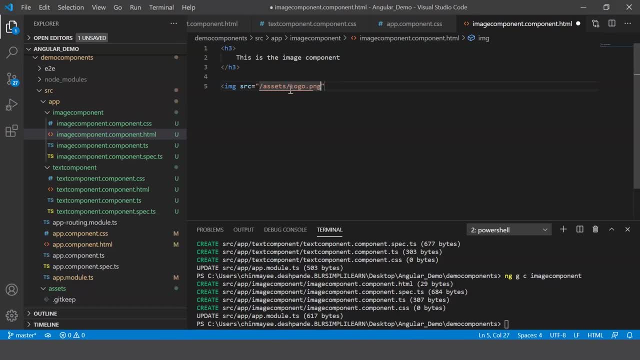 slash logo dot png. And class equals center. You can also head to your CSS file and provide any sort of styling that you need. So let me just say text align to be center, And then let's create a styling for the image, And here I mentioned the code for the image. 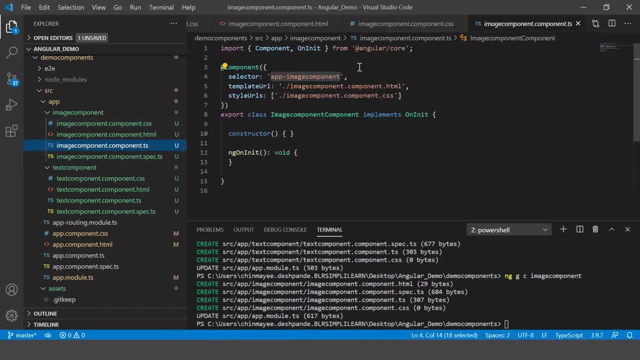 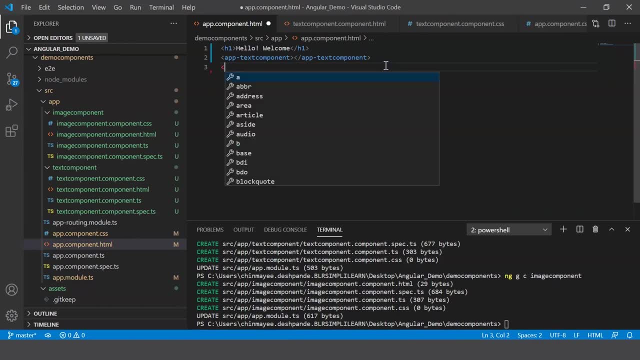 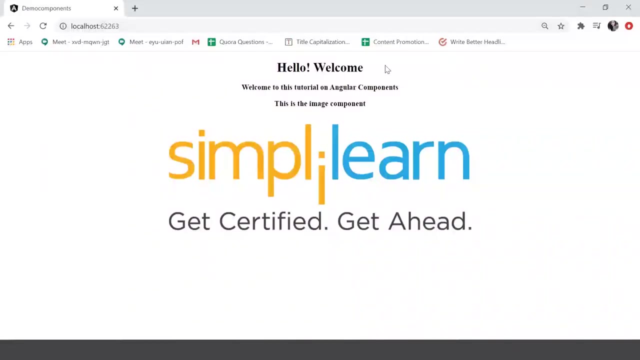 So let's save this from the dot CSS file, Let's copy it, the selector, and create a custom HTML tag in our final componenthtml file. so there we go, let's save this and check the output. and there we go. first, the hello welcome message is displayed. next, you have the message displayed from the: 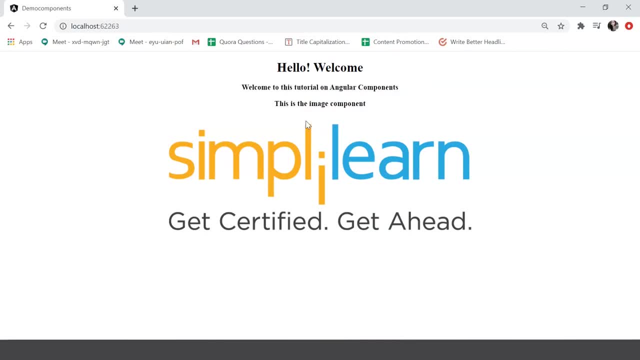 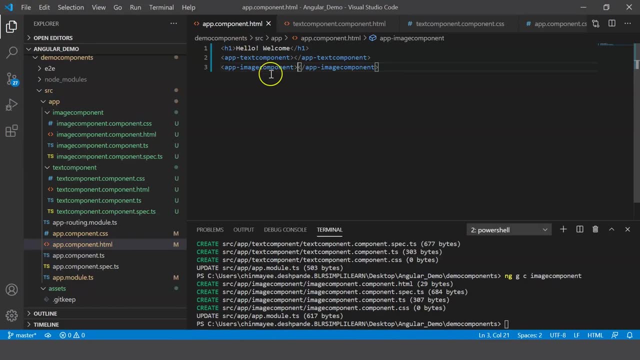 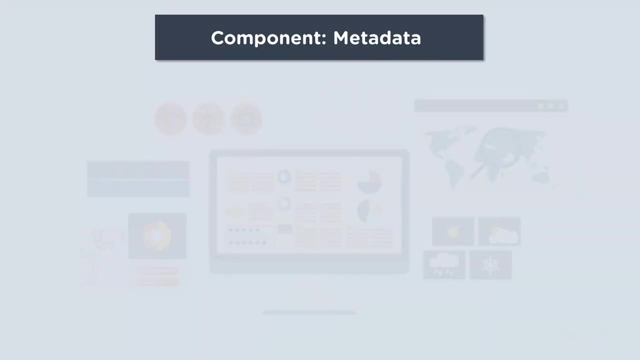 first component, and then you have the second component. so this is how you can create your own components, and don't forget to incorporate these selectors into your final HTML file. so moving on to our next topic: component decorator- metadata. now, as mentioned earlier, the at component decorator accepts a metadata. 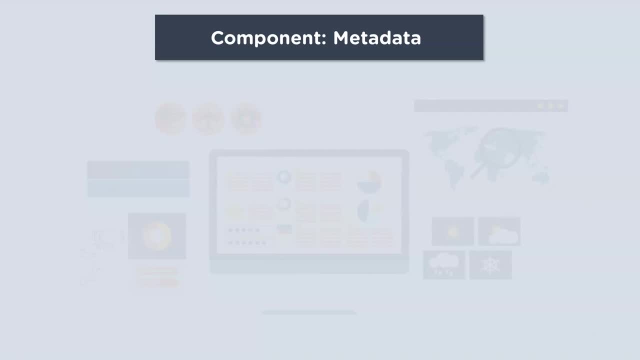 object that provides information about the component, correct? here is a list of properties of the metadata object. first up is the selector. now, basically, the selector is a CSS selector that I cream. you name the keyword and click onOK, and it identifies this particular component in a template. now this corresponds to the HTML tag, that is. 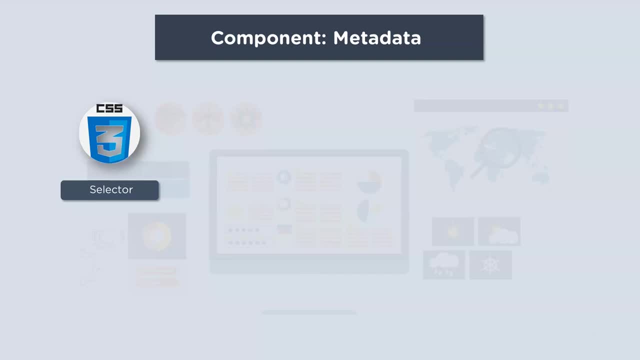 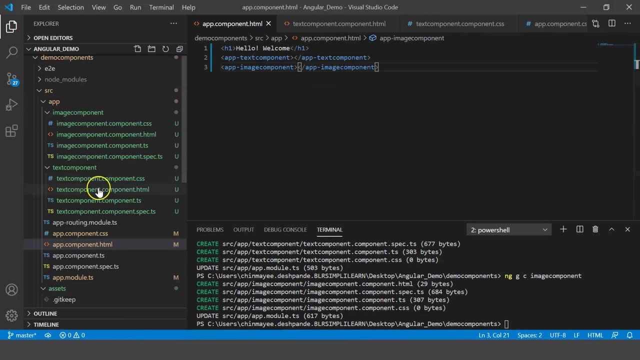 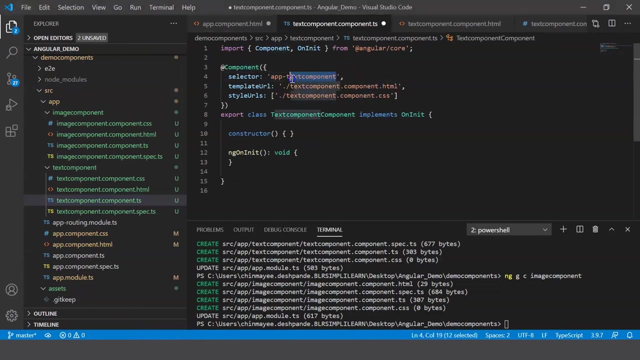 included in the parent component. you can create your own HTML tag. however, the same has to be included in the parent component. so to help you understand that better, let's head back to our VS code and say, for example, in our text component- here the selector says text component- 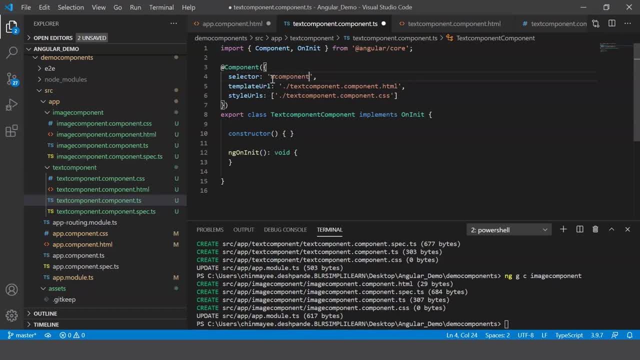 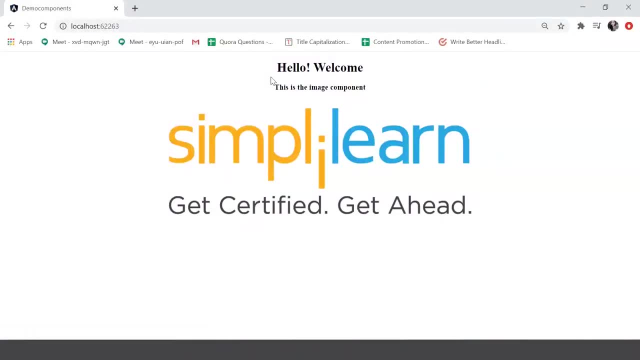 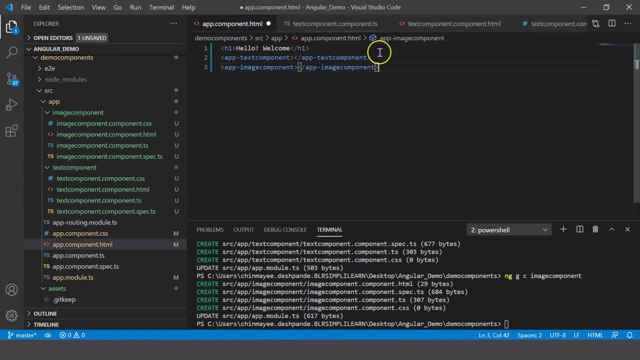 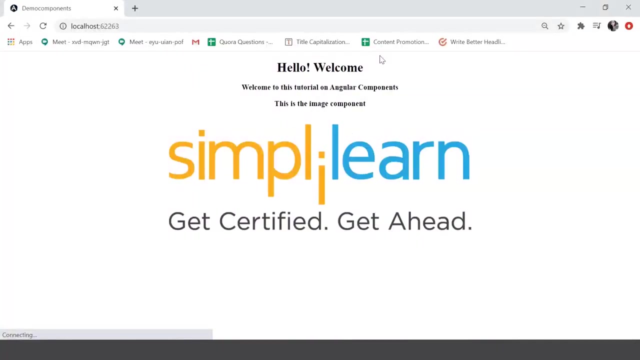 correct N component. alright. Now, when you save it and look at the browser, the message is not displayed. So what we can do is you can copy this selector and then include this here And now. you can see that the same component has been rendered onto your output. alright. 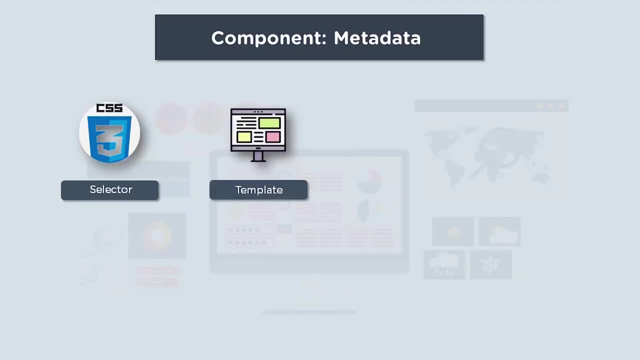 So the selector plays a crucial role in that. Next up, we have the template. Now a template is an inline defined template for the view. Now the template can be used to provide some particular markup. The markup could typically include some headings or paragraphs that are displayed on the UI.